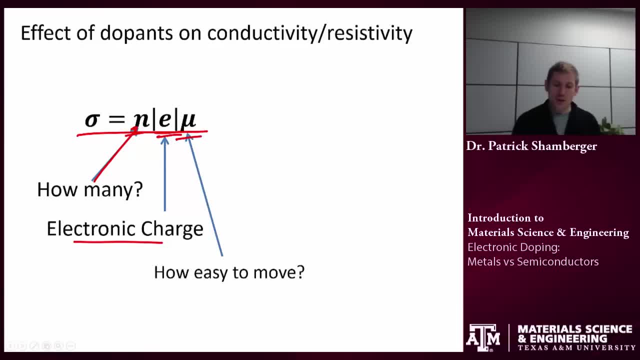 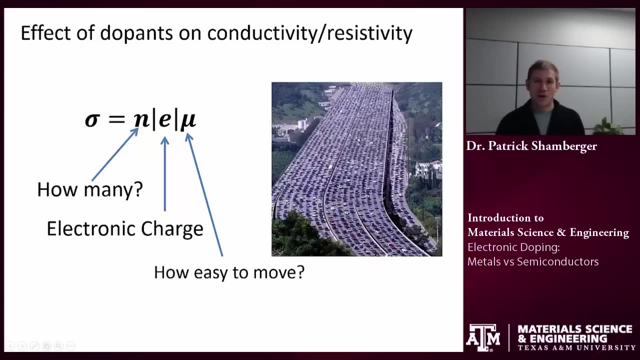 electronic charge of the free carrier. And finally, mu, the mobility. How easy is it for these carriers to move around? So if it's very easy, then I get a lot of motion and the overall conductivity can increase. Now I want to think about this in terms of an analogy, And we're 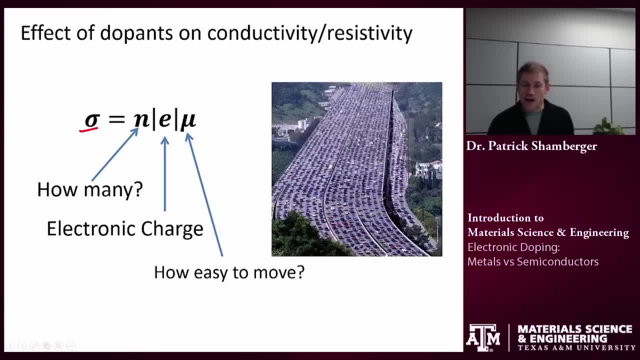 going to think about how many people are able to move down that highway per unit time. So that's our conductivity in this case. So it's going to be a function of how many cars are on the highway right. If we're in rush hour, we have a very large number of cars available. How many passengers per vehicle? 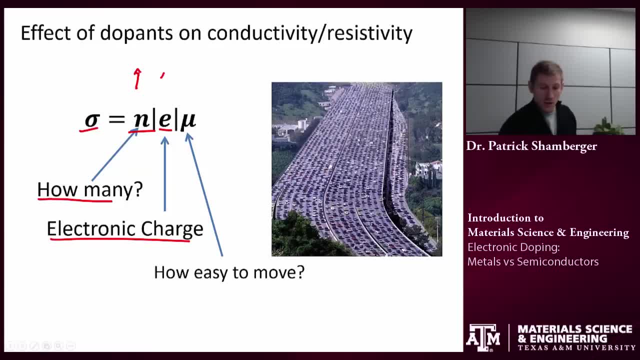 are there. If there's only one person in each vehicle, this would be, you know, one we could consider. if we want to move more people down that highway, we could consider increasing the density of passengers per vehicle And finally, mu the mobility. How easy is it for these cars to move So in this traffic? traffic dense. 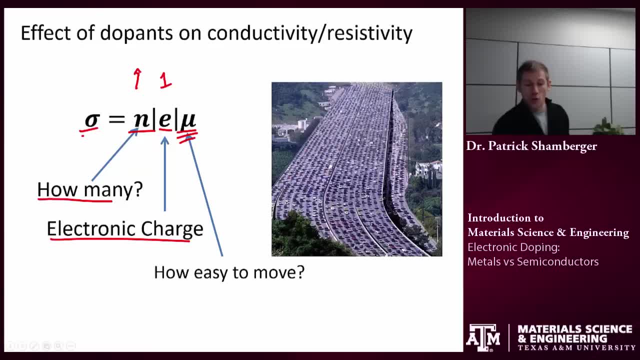 highway. the mobility is going to be what's going to control the overall conductivity right, Think about if you're driving in LA or maybe in New Delhi during rush hour. In these cases, those cars are going to only inch along right. The mobility of each vehicle is going to be very low And that 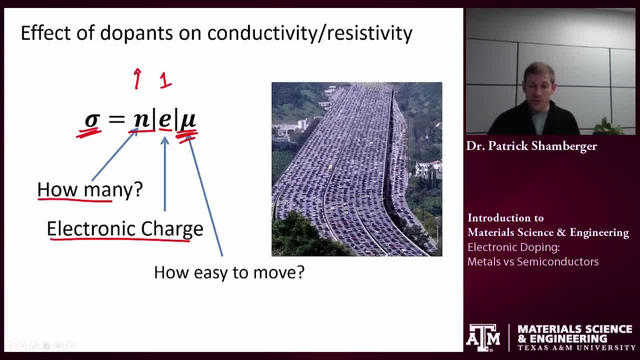 means the total number of passengers, the total number of people in each vehicle is going to be very low And that means the total number of passengers, the total number of people, uh per time moving down that highway is also going to be small. Now think about maybe an hour. 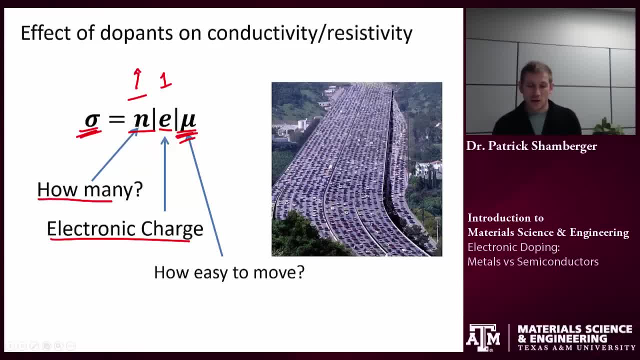 later I might still have a large number of cars on that vehicle, but the traffic is cleared up, So the mobility um is now higher, they're able to move faster and I get a much larger overall flow of people down that highway. Let's think about the other N member right. Let's think 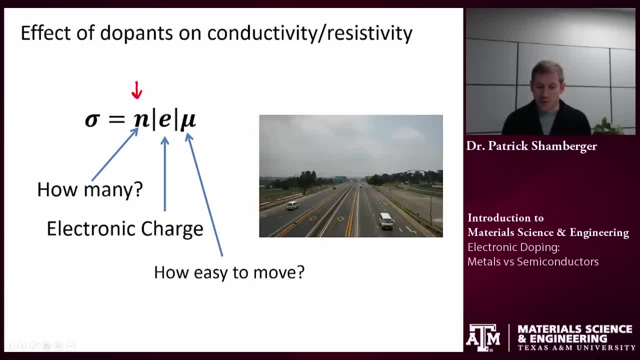 about a highway that's relatively empty, So N is a very small number In this case. um, the total number of people down the highway. uh, you know, there's not. there's not really any traffic to consider, So the mobility is probably going to be about the speed limit on whatever that highway is. 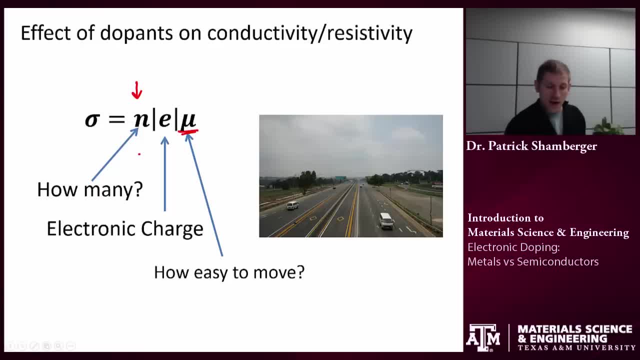 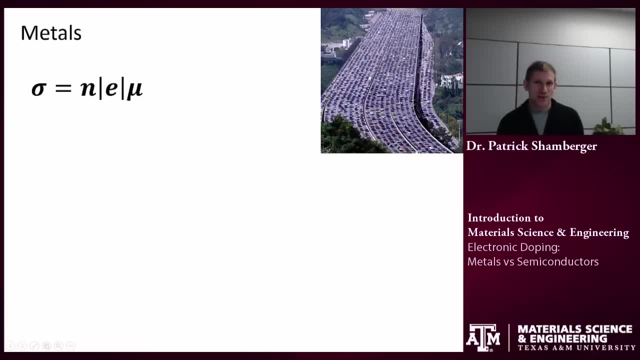 If I want to increase the number of people flowing down that highway, I want to focus on N, I want to focus on putting more cars onto that highway. So I use this analogy because it's a very good description of the two N members of the metal. 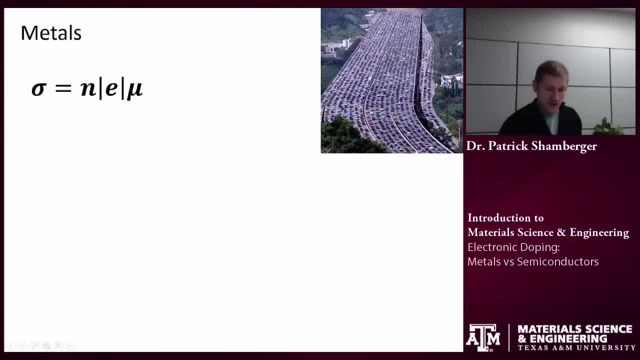 and the semiconductor case. So let's think about metals first. Metals, if you remember, um, I have enough electrons to partially fill an energy band, And so it's very easy to excite electrons up to higher unoccupied energy levels, uh, and allow them to conduct along. 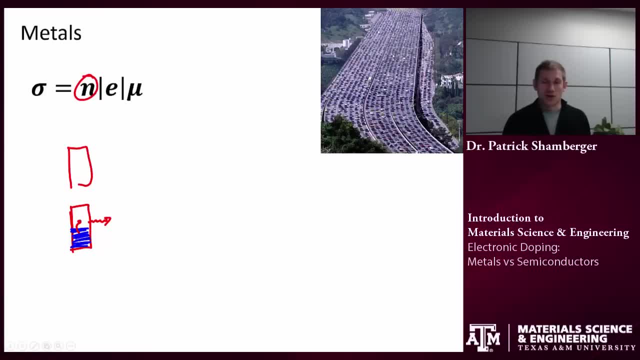 So that means N is very, very large. The number of free carriers in copper, in aluminum, in all these metals is a very large number. What limits the metals is this ability. So if those electrons are able to travel relatively easily without scattering, 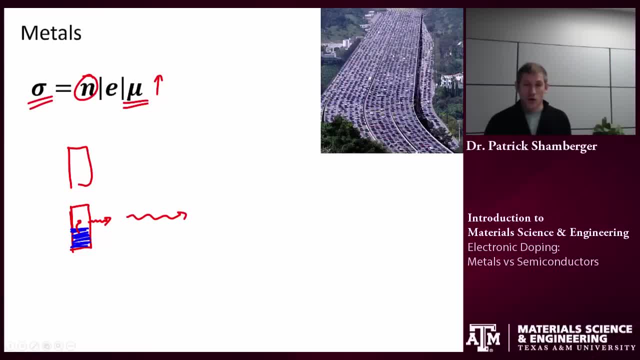 they could have a high mobility and a conductivity. overall conductivity could be high. If there's something that I introduce that's causing those um car, those- sorry, not cars- those electrons to scatter and not flow very easily, then that could decrease the mobility. 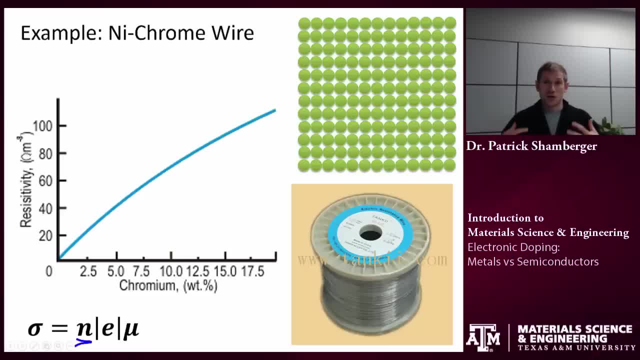 decreasing the overall conductivity, And when I talk about doping or conductivity in alloys, that's exactly what happens. So we're going to think about an example: um nichrome wire. This is a metal wire that's oftentimes used for resistive heating, And it's nice because we can. 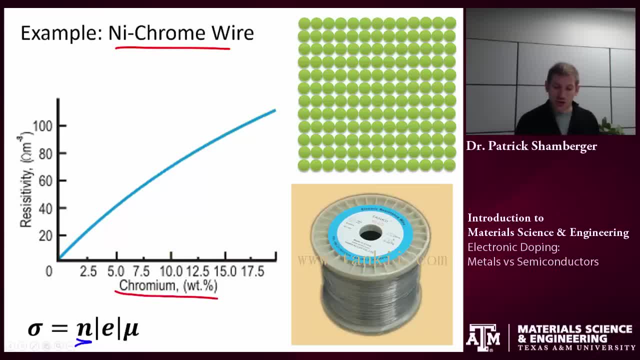 control the resistivity very easily by controlling the percent of chromium in the system. Um. so I see, if I have a pure nickel wire, my resistivity is low. That means my conductivity is high. As I start increasing the percent of chromium, in that the resistivity increases. 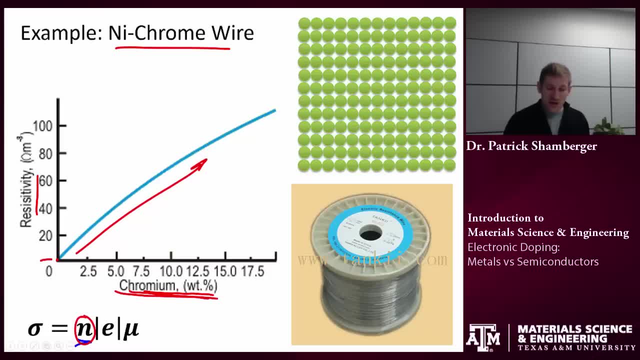 Dramatically. what am I doing? The number of free carriers does not change very much in this case. In metals, I have plenty of free carriers. That's not the limiting factor. The limiting factor in the metals is this mobility, that traffic density, right. So if I start thinking about a picture of 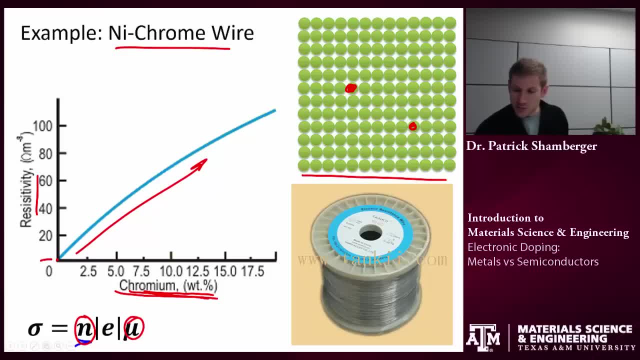 pure nickel and let's start introducing some chromium defects. you know the electrons are moving along, they're flowing, but when they hit this defect they're more likely to scatter And that makes it more difficult for the electrons to flow through the system. The more chromium atoms I have in here. 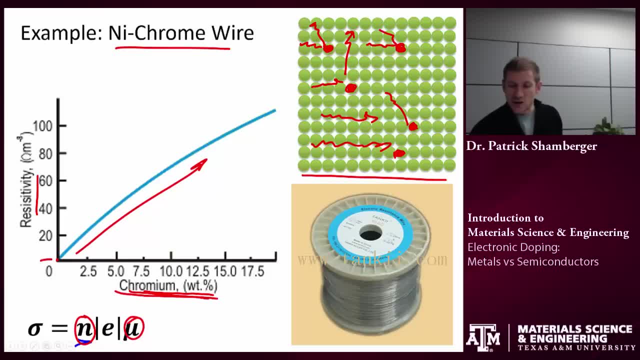 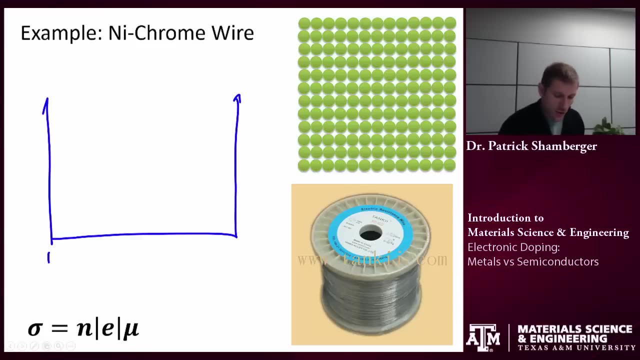 the more potential defects there are that will scatter electrons. So the result is: as I increase the chromium concentration, the overall resistivity increases. Now this is kind of weird because if I thought about a system where I go all the way from pure nickel to pure chromium, these are both metals And so their overall resistivity. 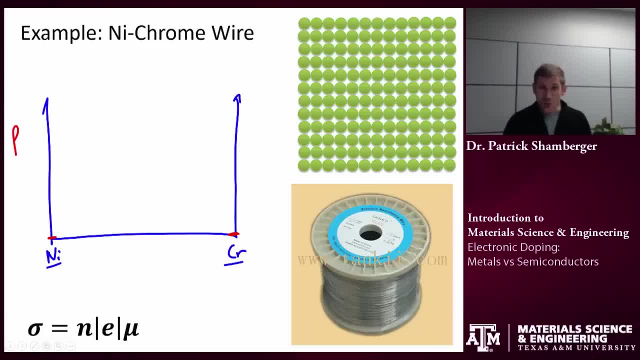 of pure nickel is quite low and the resistivity of pure chromium is also quite low, But once I start alloying it I increase resistivity dramatically. So I can't say that the resistivity of nichrome is an average A of the resistivity of nickel and any szerp of chromium. 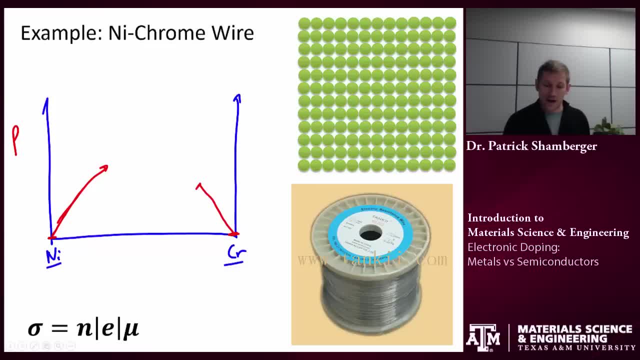 Use A to minimize resistivity of Ichromium echo, which is all of thecamp wissen g bomb. It doesn't work that way. because of this atomic mechanism, When I'm increasing the concentration of chrome in the nickel lattice, it's soluble within that nickel. 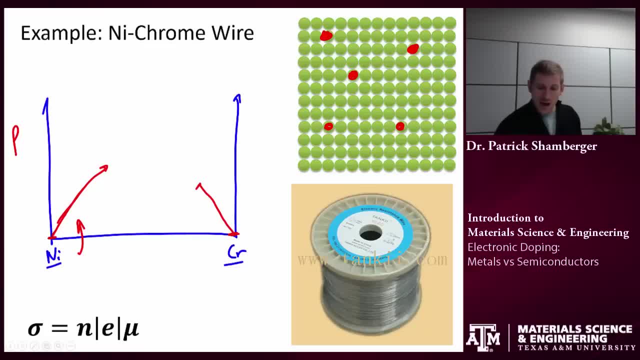 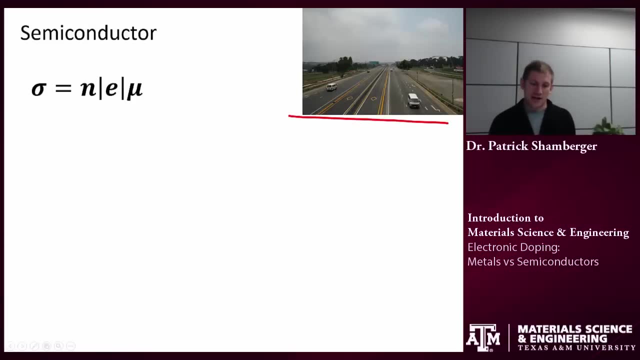 so those atoms are gonna be dispersed relatively evenly and they're all gonna be creating scattering sites. So I have to think about it on this atomic level, not this bulk mixing level. Semiconductors- the semiconductor case is this empty highway case. 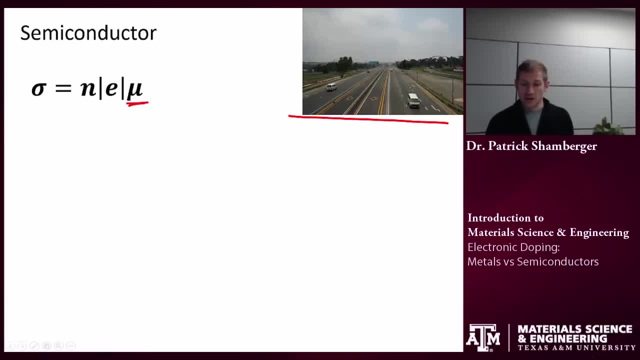 Semiconductors are largely not limited by the mobility. I can have some semiconductors that have a higher mobility than others, but the biggest thing that's gonna impact the overall conductivity is if I increase the number of cars on that highway. 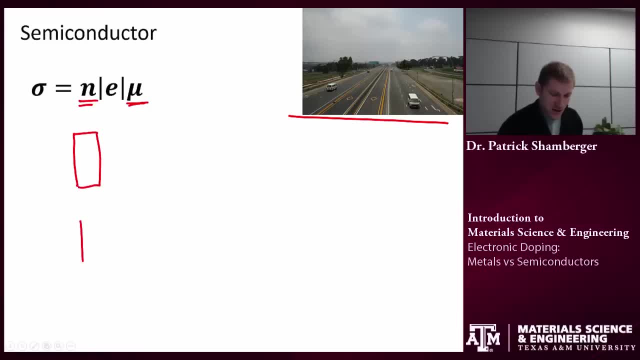 the number of free carriers. So again, remember the semiconductor picture. Here I could have my valence band and here I have my conduction band. The valence band is gonna be full and the conduction band is relatively empty, So I can increase the number of carriers. 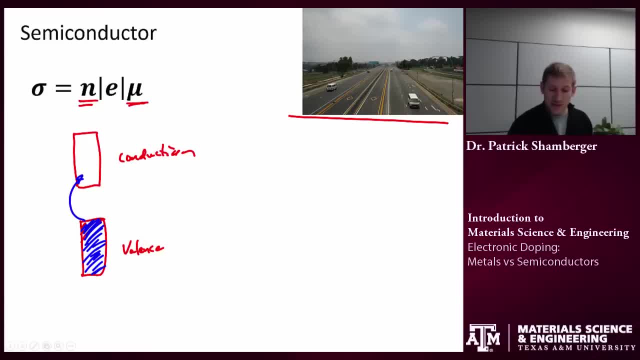 in that conduction band by one of two ways: I could increase the temperature excite more up there, or I could put dopants in, And so dopants are elements that have electrons that are very close in energy level to the conduction band. 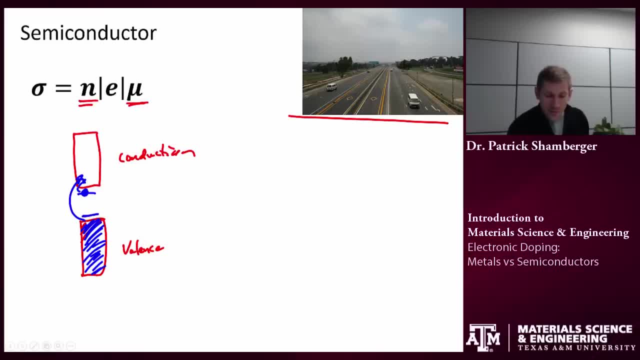 so it's easy for them to hop up there. Or maybe they're acceptors so they have available energy levels very close to this valence band so it's easy to excite and put an electron up there, In either case, in the silicon.